Hi guys, my name is Dr Arohi Manyar and today we are going to study about public health dentistry. So in public health dentistry we are going to study about the statistical test. So our statistical tests are grossly divided into two parts, that is, the parametric test and the non-parametric test. 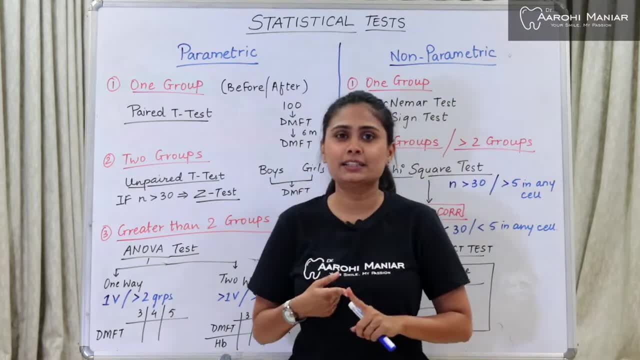 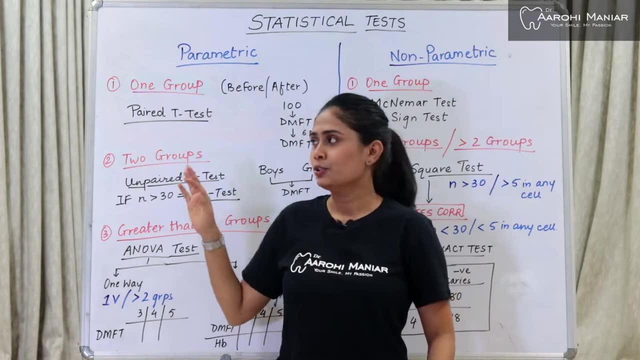 So in a parametric test we need to remember three points: that it is a quantitative test. Second, mean is taken into reference, mean median mode that we used to study. So here mean is taken into consideration. and third, in our parametric test we have a normal distribution curve. 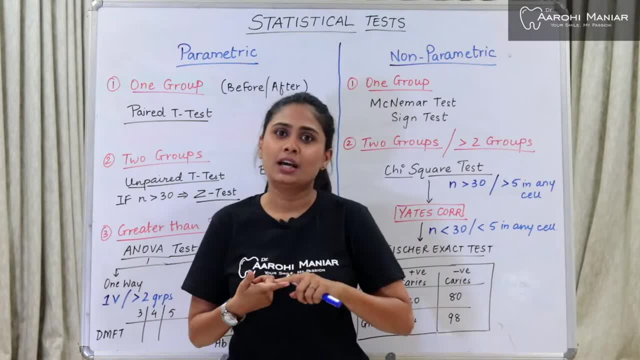 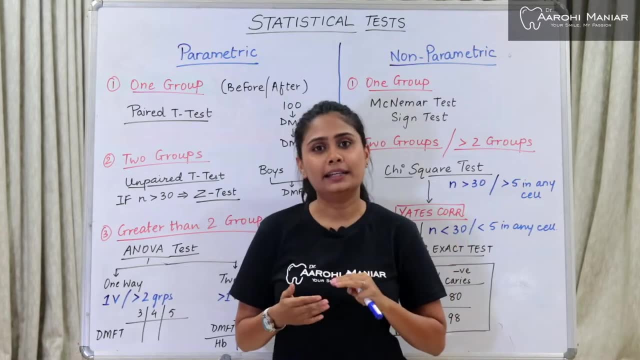 Whereas, moving on to our non-parametric test, it is a qualitative test. This was quantitative, this is a qualitative test. Here, median is taken into consideration. and the third point is: this does not have a normal distribution curve, It has a non-normal distribution. okay, 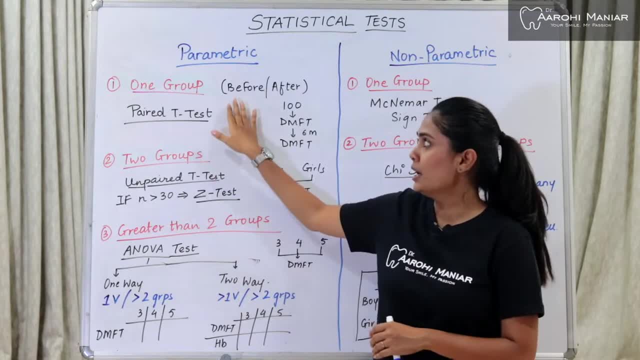 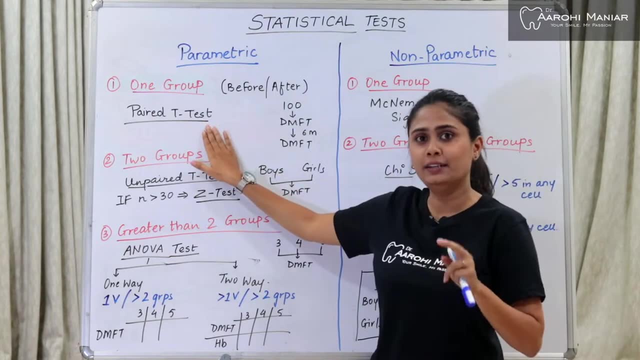 So in parametric test we have divided into three parts. When we have one group of people or one group On to which we have to perform our test, we perform our paired t-test. So how to remember this? So whenever we have a before- after kind of a situation, 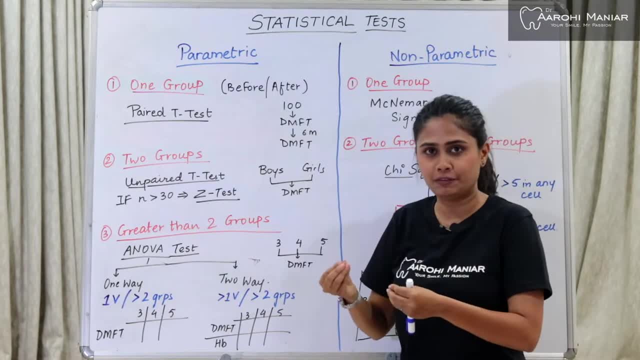 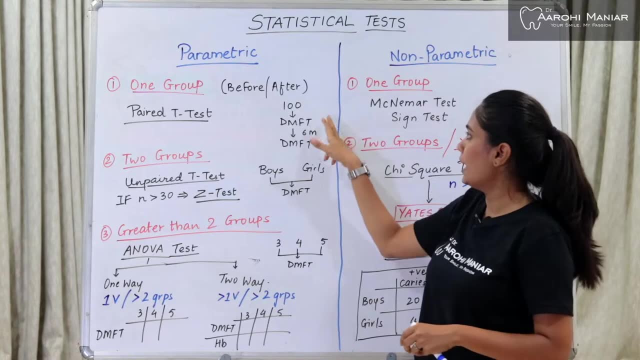 I have a group of people on which I have to perform my DMFT index. So I have- let's say I have- 100 people, So it's that is one group In 100 people. I have to perform my DMFT test before and after. 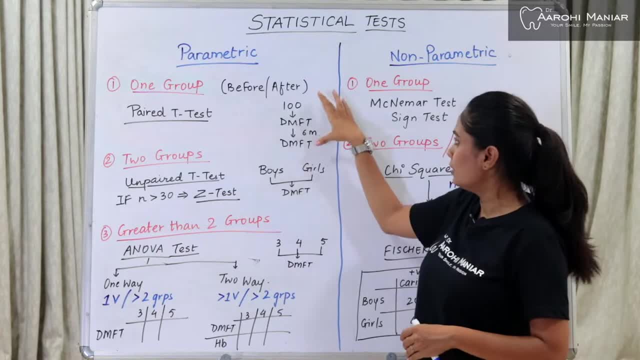 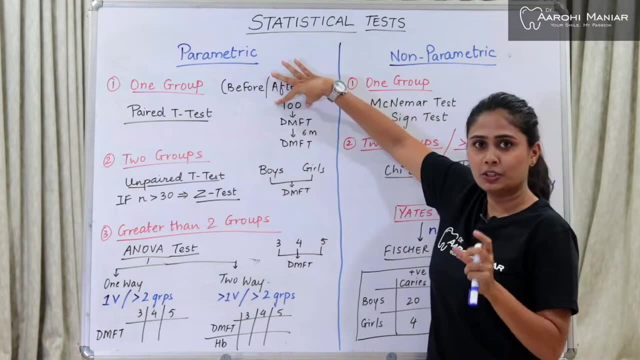 So this is before six months, this is after six months. So these kind of before after situations we go about with our paired t-test because the group is same, The group of choice or the group of population is one, It is only one group, it is the same. 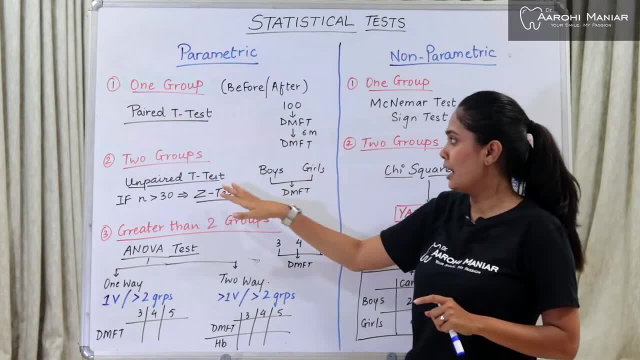 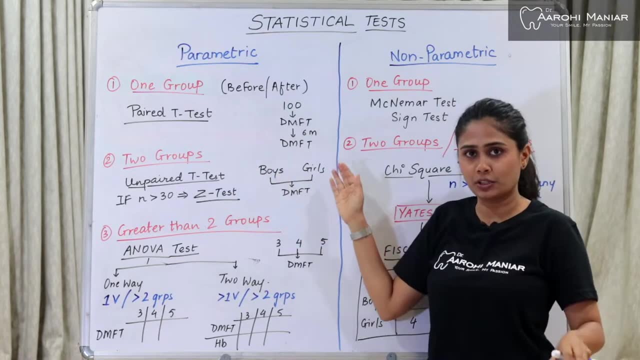 On the same people. we are performing this test. After that we are going to two groups. okay, So when we have two groups, for example, when we have a group of boys and we have a group of girls, When we segregate into two groups and then we take DMFT index, 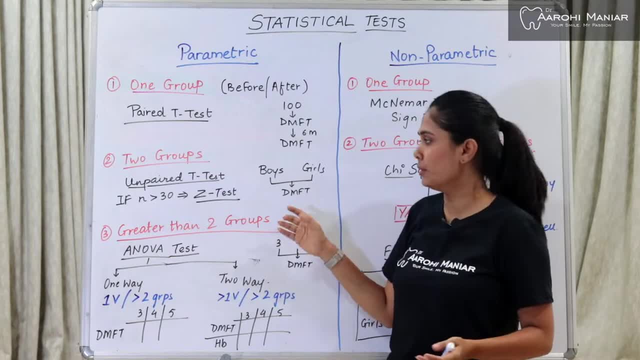 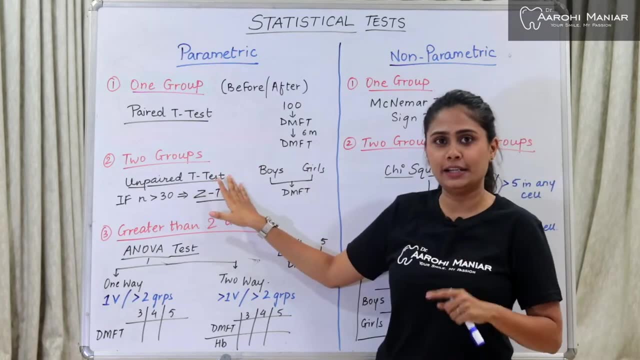 This can be any index. This is just taken for example. So when I separate these two groups, So when I separate these two groups, I can separate these population into two groups, and then I take a test. It is known as unpaired t-test. 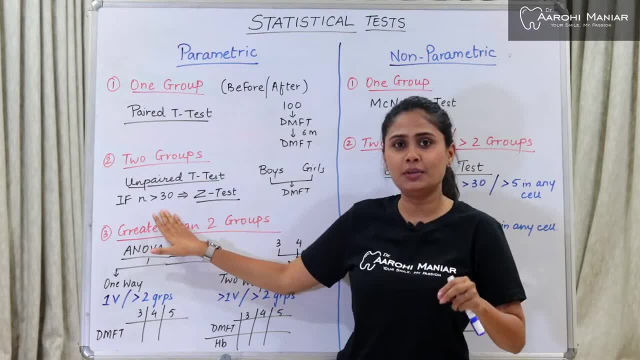 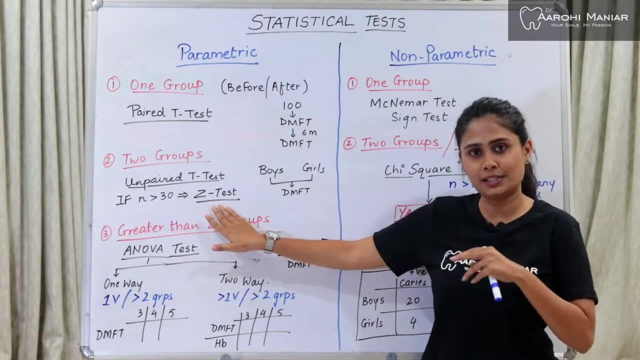 So in such cases, when N is greater than 30, N means my group of choice, So when the group of choice in the group of choice is greater than 30. The test itself is known as Z test, Moving on further to greater than two groups. 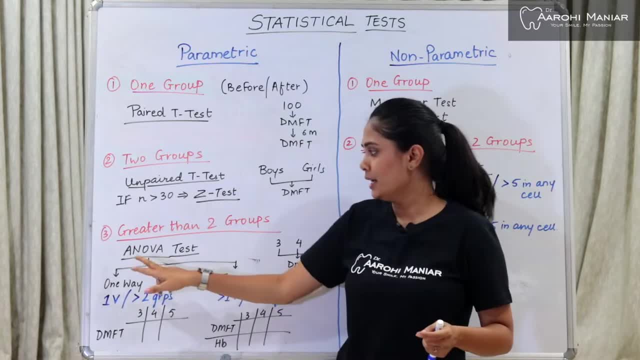 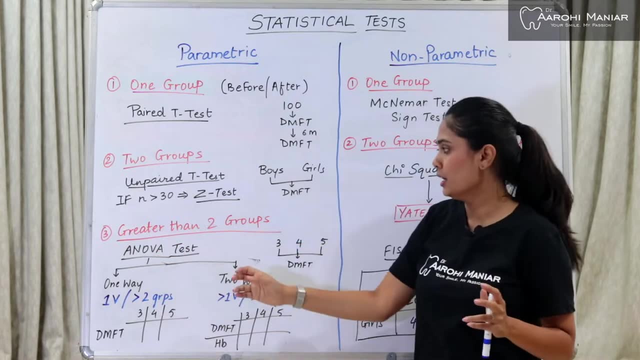 We have ANOVA test. What does ANOVA test mean? It is analysis of variance. This is just a short form. The whole thing that means is analysis of variance. The whole thing that means is analysis of variance. So in this again we have two different types. 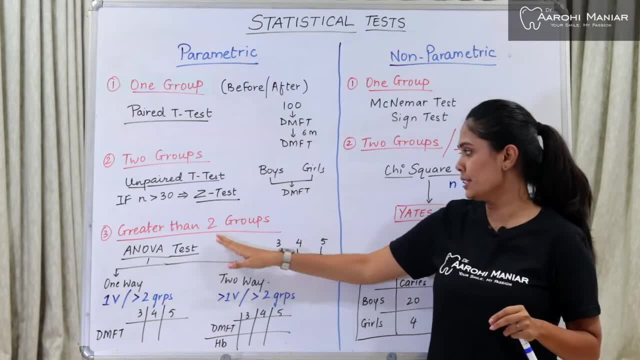 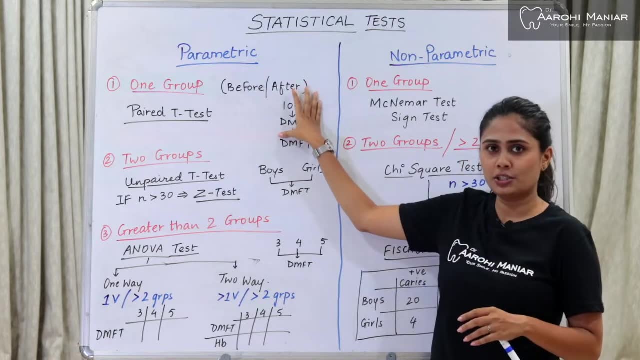 So the first thing that we have to remember about ANOVA test is we have greater than two groups. So here I have three years, four years and five years. This I have divided. first I had just one group, then I divided into two groups, that is, boys and girls. 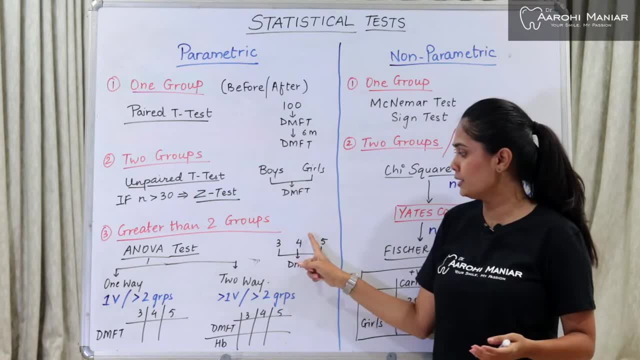 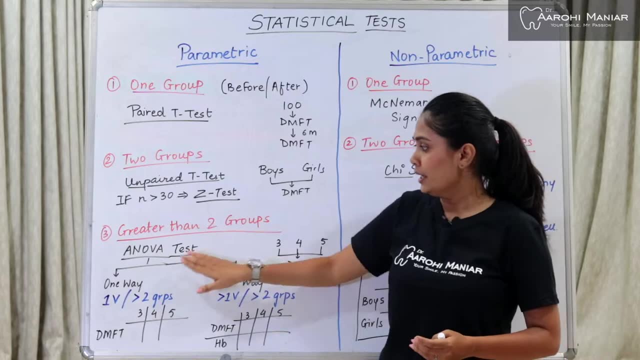 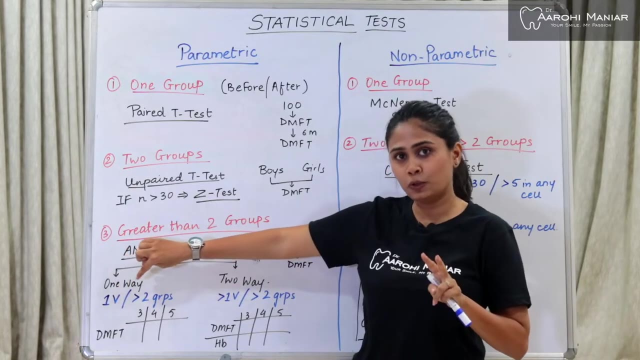 Now I am dividing it into age wise- three years of age, four years of age and five years of age- and then I am taking my DMFT index. So this is our ANOVA test, The one way ANOVA. this is one of the types, the one way ANOVA test. in this there is only one variable, but there are more than two groups. 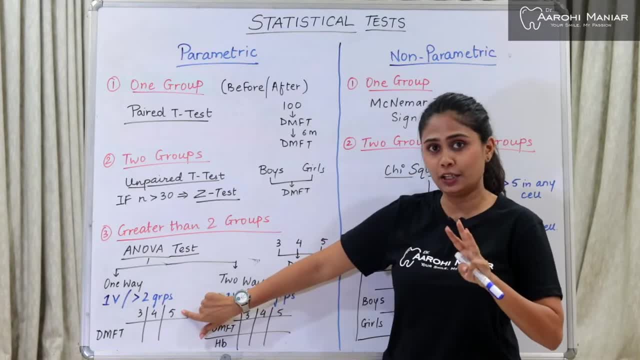 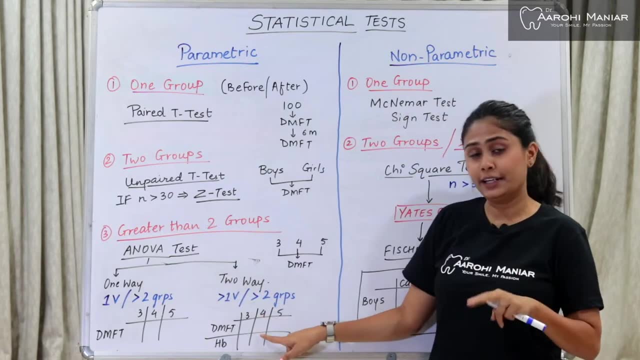 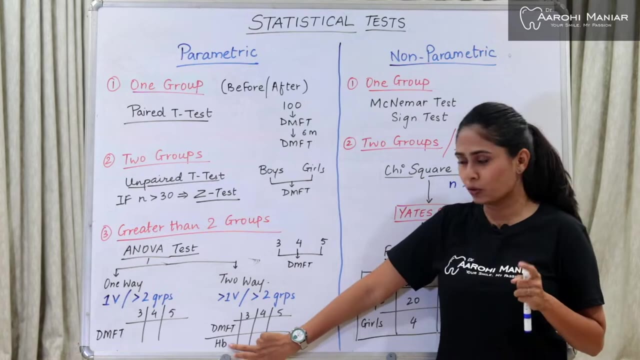 So this three, four and five years, these are more than two groups, these are three groups and my variable is only one, that is DMFT, Whereas in two way ANOVA I have greater than one variable and greater than two groups. So I have DM. I am also taking DMFT along with the hemoglobin. 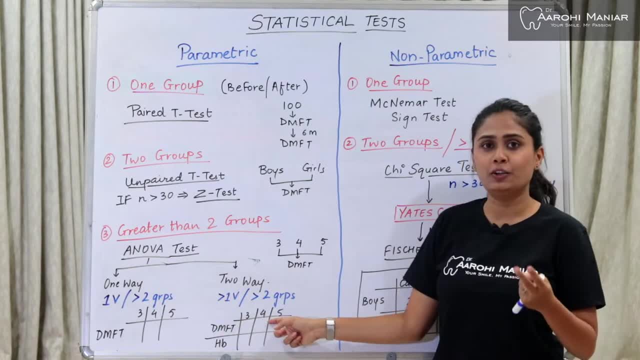 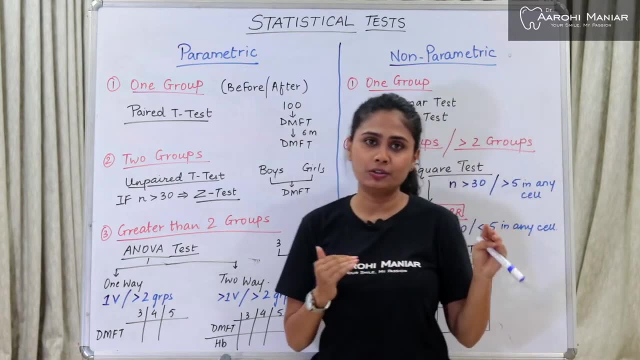 So these are my two variables, and it is in greater than two groups, That is, here I have three groups, it can be four, five or multiple. So that is all about our parametric test. moving on to the non-parametric test, 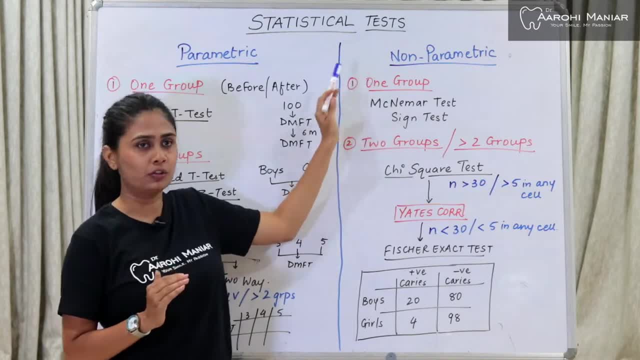 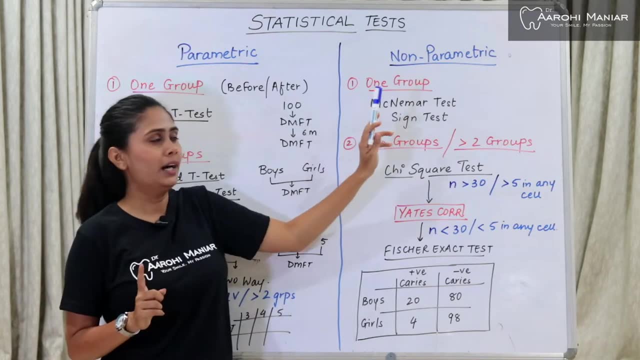 So it is a very simple thing here. Here we only divided into one groups, two or greater than two groups. ok, So if I have, I am performing a non-parametric test on one group. I call that test known as a Mach-Nema test or a sign test. 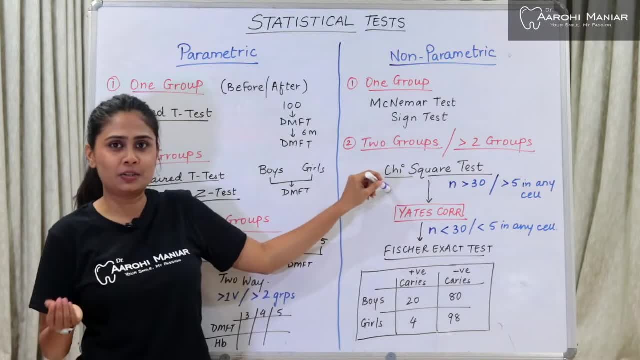 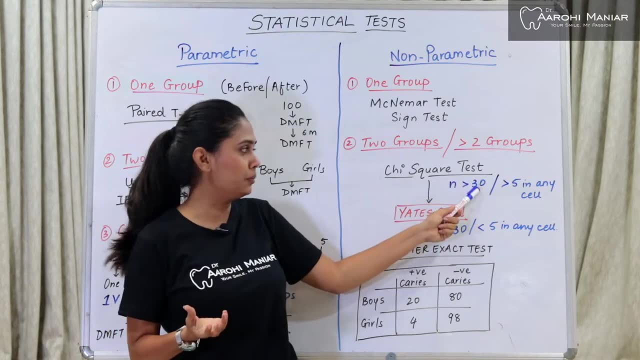 For greater than two groups or two groups, something known as chi-square test or chi-square test. Whatever you People want to say here. the population, the group which I select- should be greater than thirty and there should be, the number should be greater than five in any cell. 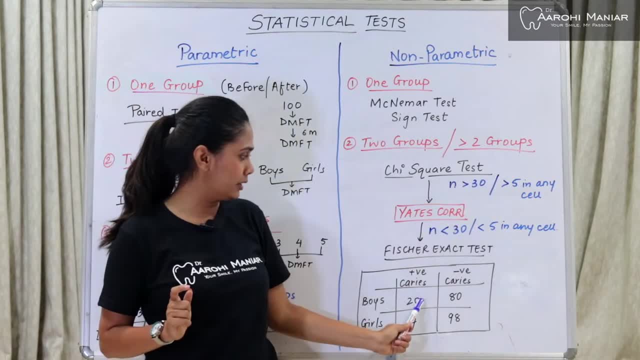 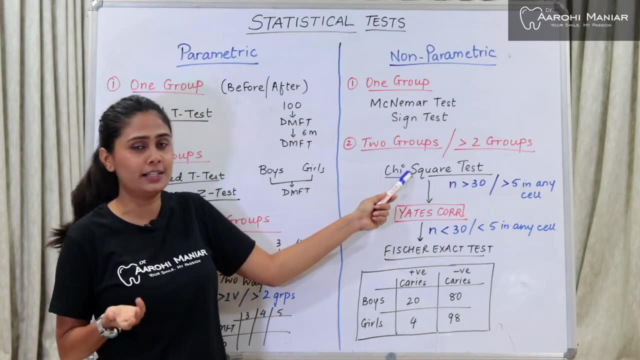 So this is my group here. it should be greater than thirty. this is ninety, this eighty and ninety eight. this is greater than thirty, but these two are not greater than thirty. So this cannot be called as chi-square test. So somebody known as somebody called it as a Yates correction. 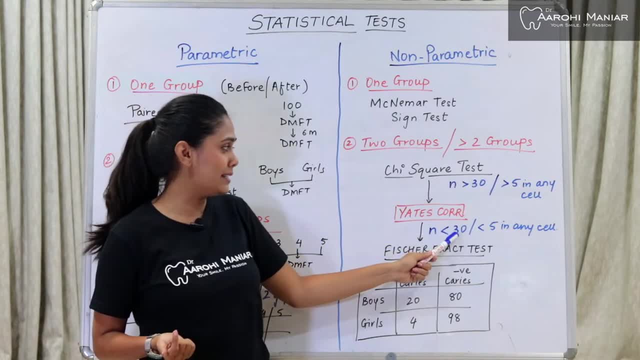 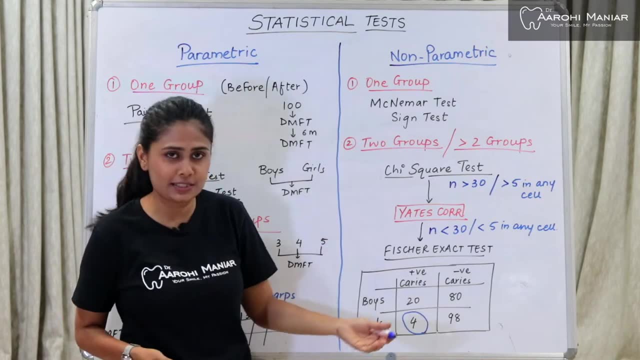 So what happens in Yates correction is when the N is less, So somebody known as somebody called it as a Yates correction. So somebody is more or less than thirty, like here, or when there is less than five in any cell. So if this is less than five, four is less than five, obviously. 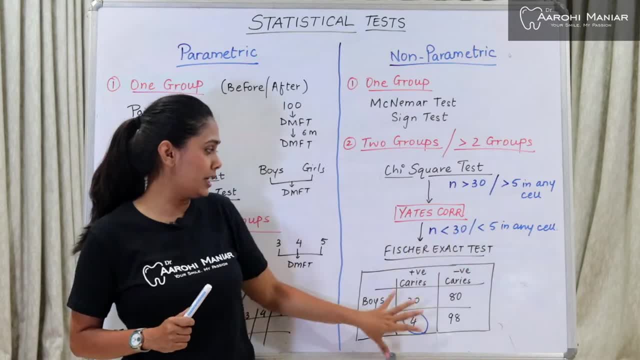 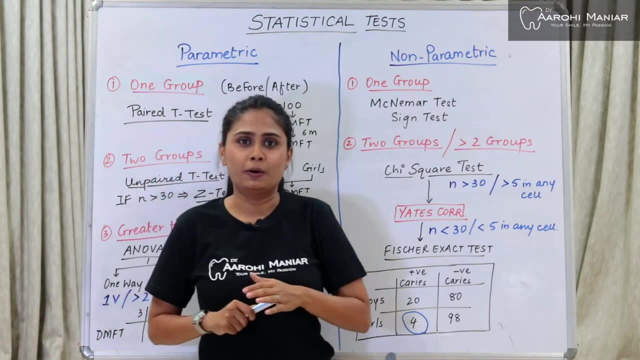 So in one of the sales we have less than five number. So such kind of cases can be solved with our Fisher exact us. So that is all about our non-parametric test. So I hope you guys enjoyed this video and that is all about the statistical test in public health dentistry guys. 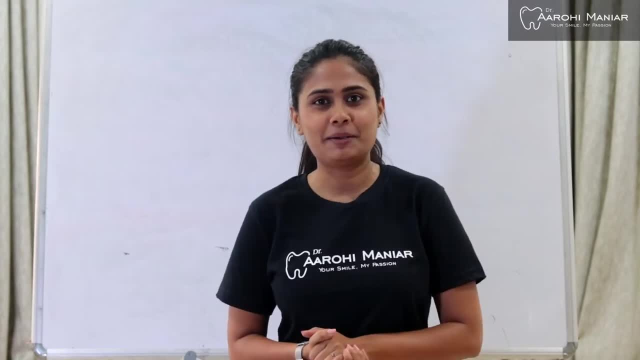 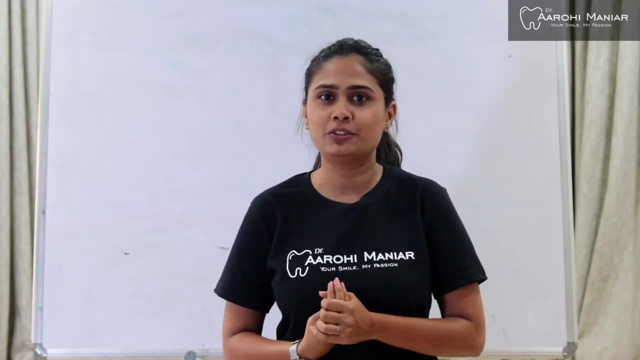 I hope you like this video. Please hit the bell I can and subscribe to my channel for the upcoming notifications. also, don't forget to comment in the comment section below about the topics that you want me to discuss later on and to get in direct touch with me. you can also dm. 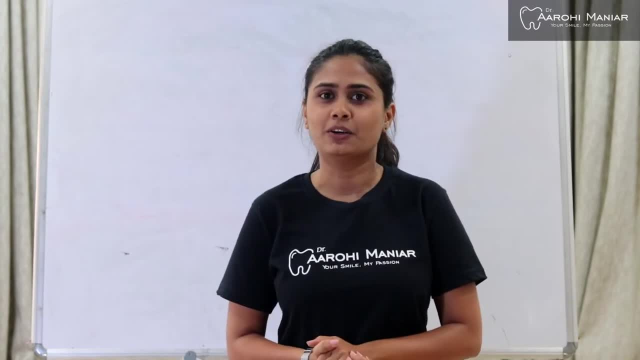 me on my instagram id, which i'll be putting in the description box below. thanks for watching. 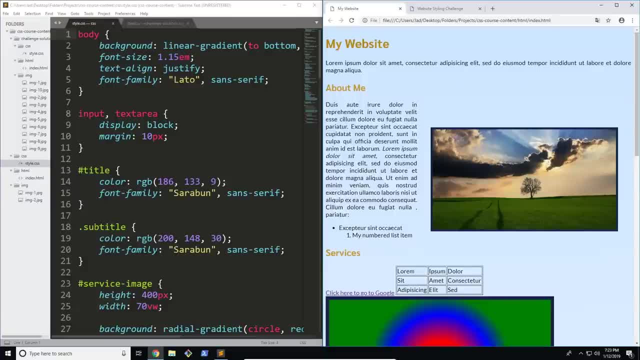 Hi, welcome to the CSS zero to hero course. In this course, you're going to completely learn how to use CSS from the ground up. We're going to cover every single concept or every major concept in CSS and really build up our knowledge of it. So before we move on, I just wanted to 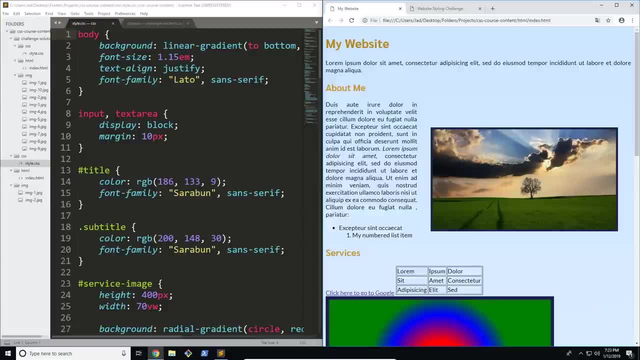 give you some motivation on what you're going to be doing in this course So you can really get excited about the course and start jump- you just jump- straight into learning. So first of all, let's look at some of the stuff that we've done over the course. Now we start with a base website. 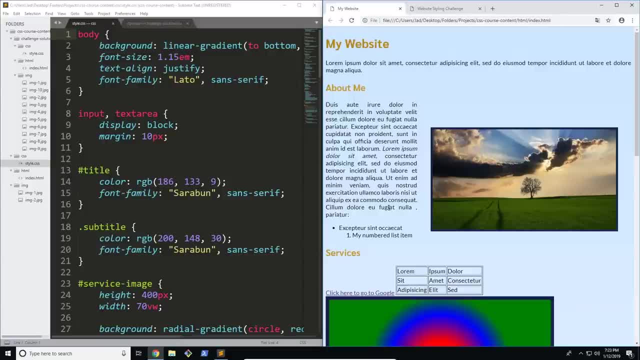 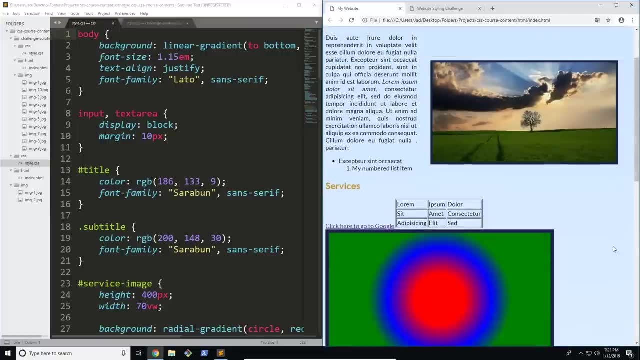 and over time, we style this and change up the website using every technique that we've learned. So you can see that we've created multiple grids, colors. we've changed this completely and transformed the website in every single way. We've also created things like gradients. 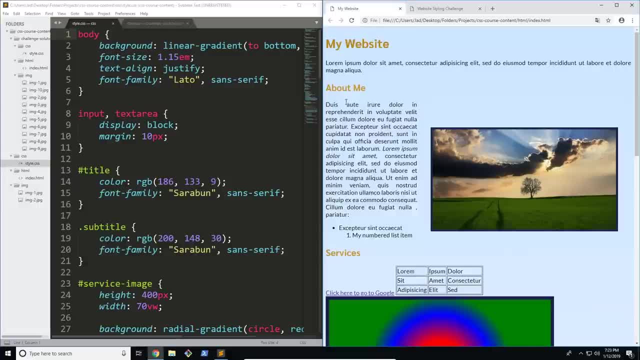 and we've also styled, changed our custom fonts, colors, and we've also created a lot of different things like gradients. We've also created things like gradients and we've also styled, changed our custom fonts and backgrounds. We cover all of this in depth throughout the course and we do it step by step. 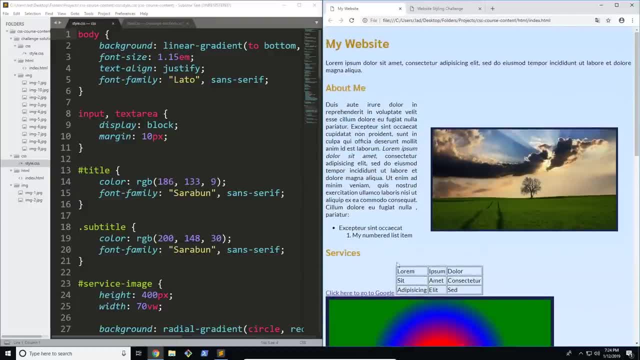 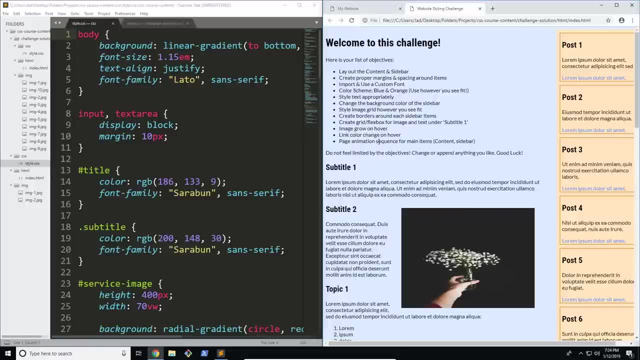 so that you don't rush through and forget anything At the end of the course. there's also a little challenge here, where you try to bring all your skills together and style the website from scratch. Now there is a solution video if you need it. Maybe you just want to see.